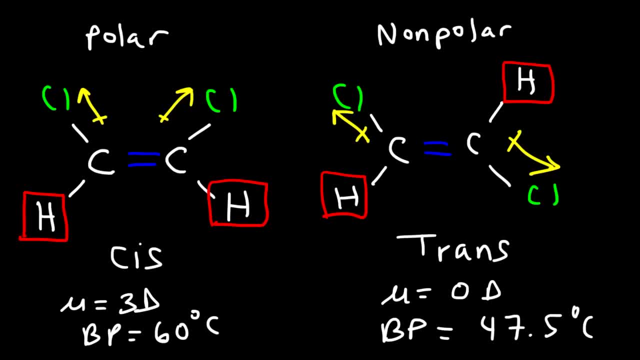 about 47.5.. So polar molecules typically have a higher boiling point than nonpolar molecules. As you can see, the cis and trans isomers have different physical properties. They have different boiling points and different dipole moments, and this is due to the fact that the double bond 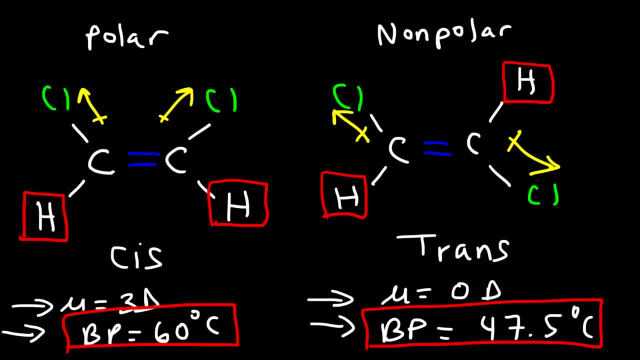 lacks a dipole moment. So if you draw the dipole moment on the left, the dipole moment is greater. when the cis isomer is between the red and the bottom, The dipole moment has a higher boiling point in the bottom. If you draw the dipole moment on the green or the blue, you can see that the dipole 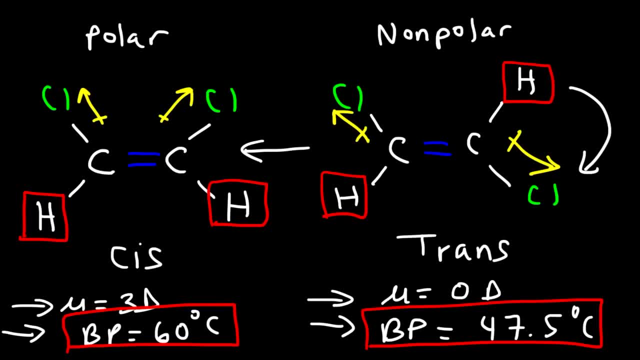 moment has a higher boiling point and you can see the dipole moment is higher when both are in the top. And if you look at the right, you can just see that if the dipole moment is between the green and the bottom, then you can see that the dipole moment is greater and you can see the dipole. 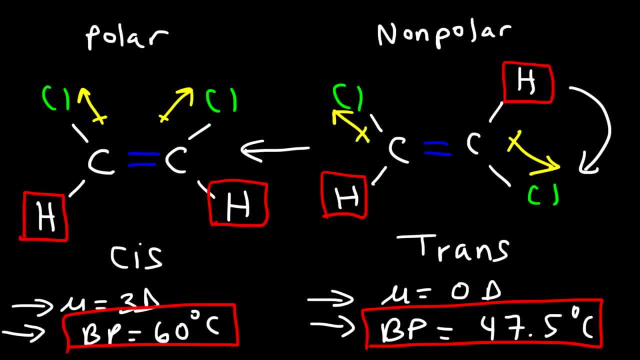 moment is greater And that's why you have such different physical properties. In the case of ethane, you do have free rotation among the carbon-carbon single bond. The energy barrier is isomers. the energy barrier is very, very high, so it takes a lot of energy to break. 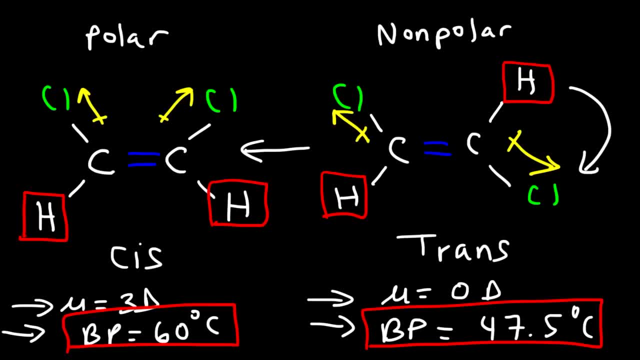 that pi bond, and so these are two distinct isomers with different physical properties. so it takes a lot of energy to go from the transform into the cis form, and so there's no free rotation with cis and trans isomers. it takes a lot of energy to convert from one form to another. now there's different ways to. 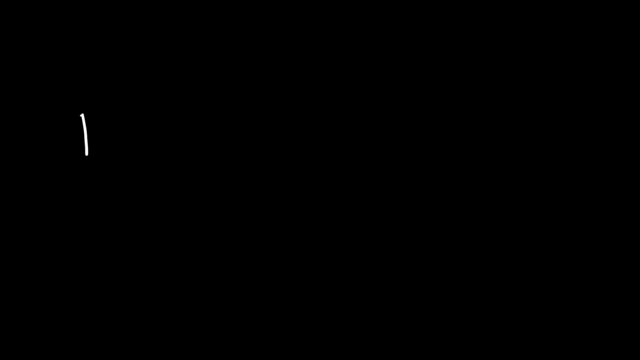 represent cis and trans isomers. you can also represent them using rings. in this example, we're going to have two hydroxyl functional groups on the wedge, so that is going out of the page, and on the right we're going to have one on the dash which is going into the page and one on the wedge. 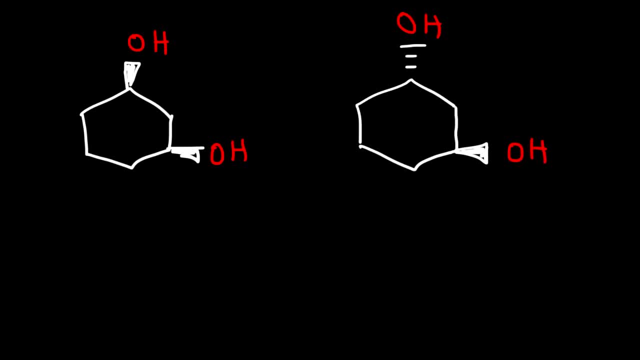 so on the left we have the cis isomer, because both hydroxyl groups are going in the same direction. out of the page. on the right we have the trans isomer. one is going into the page, the other ones going out to the page, so one is going up. 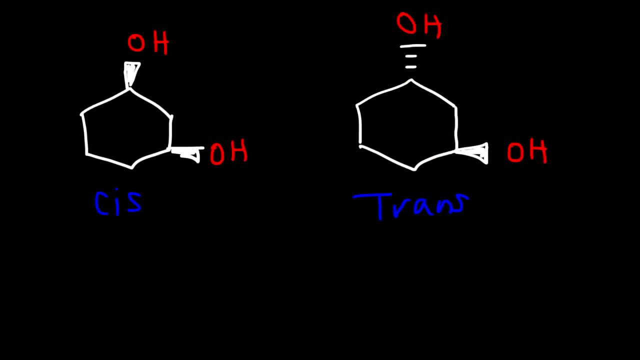 the others going down, and so they're in opposite directions, and so that's another way in which you could represent cis and trans isomers. now consider these four molecules. so what I want you to do is determine which of these alkenes can show cis and 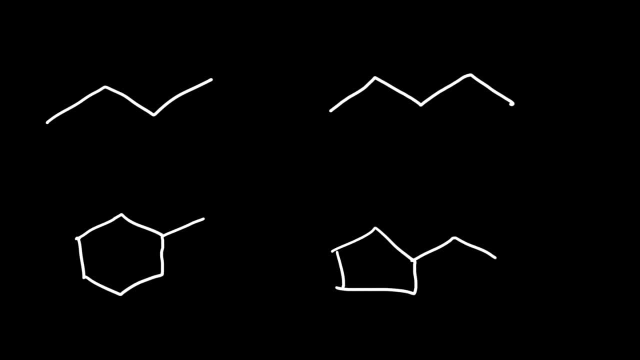 trans isomerism. so which of these molecules can you draw cis and trans isomers for? so let's look at the first example on the left. can we draw the cis and trans isomer for this alkane? it turns out that we can't, because on the carbon. 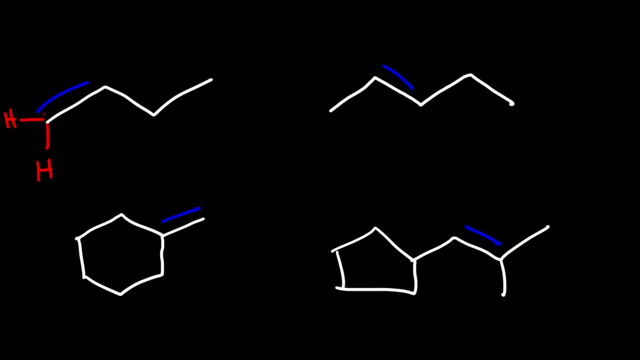 at the left. it has two atoms that are the same. so if the two groups are the same, you can't show cis and trans isomerism. for this one you could. this is the trans isomer, so this carbon is attached to two different groups. it's 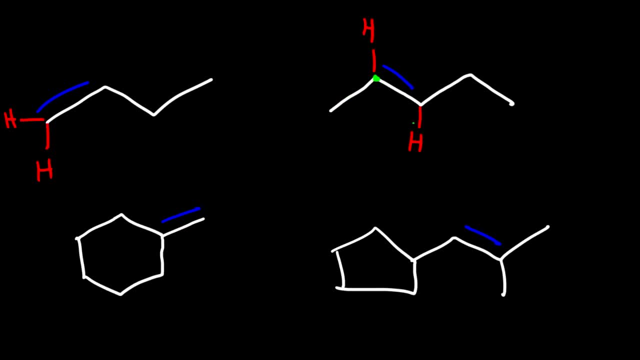 attached to a hydrogen and a methyl group, and this carbon is attached to two different groups: hydrogen and an ethyl group. so what we have here is the trans isomer. so if you want to draw the cis isomer, we can draw like this, and so notice that the hydrogen atoms are facing the same side. so that's the cis. 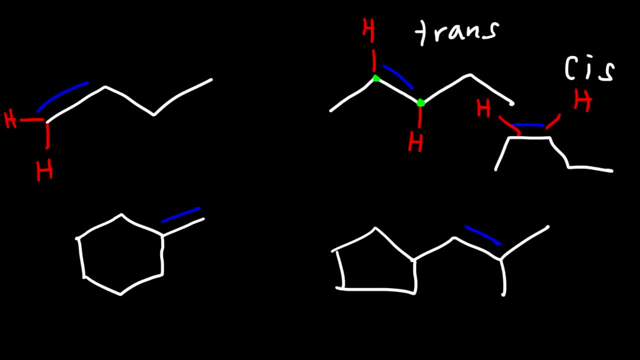 isomer for this particular alkene. now for the third example. we can't show any cis or trans isomers because this carbon is attached to the same group. it doesn't have two different groups attached to it. the same is true for the last one. this carbon that's part of the double bond- is attached to two methyl groups. so 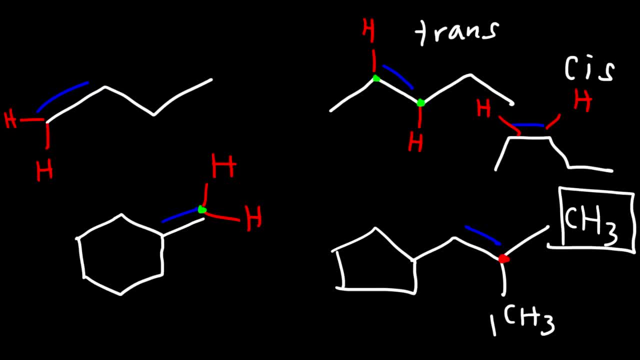 because these two methyl groups are identical to each other. this alkene doesn't have any cis or trans isomers, so the only one that has it is this example. so that's how you can tell if an alkene will have cis and trans isomers. look at: 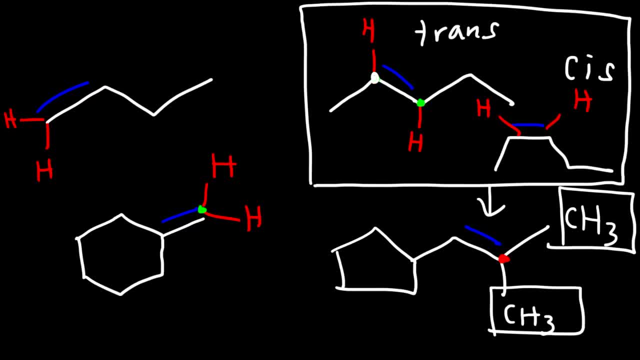 each carbon that is part of the double bond and analyze them, see if they're attached to two different groups or if they're attached to two of the same group.